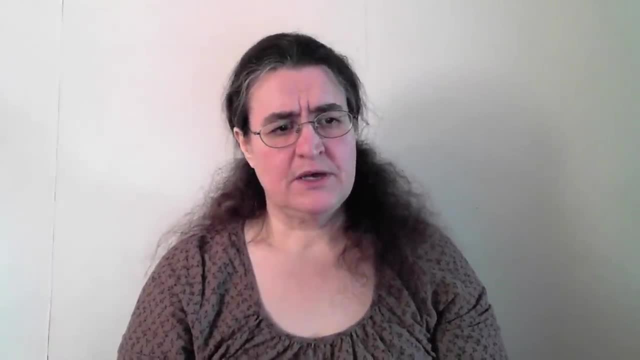 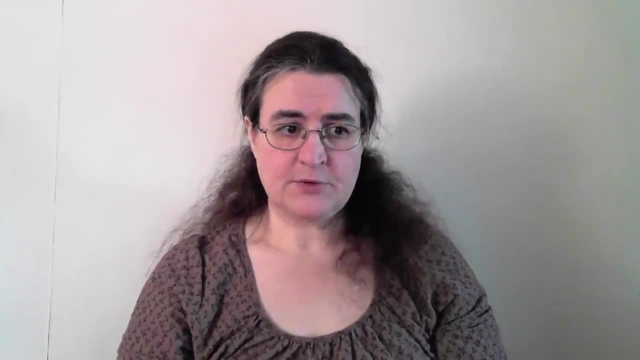 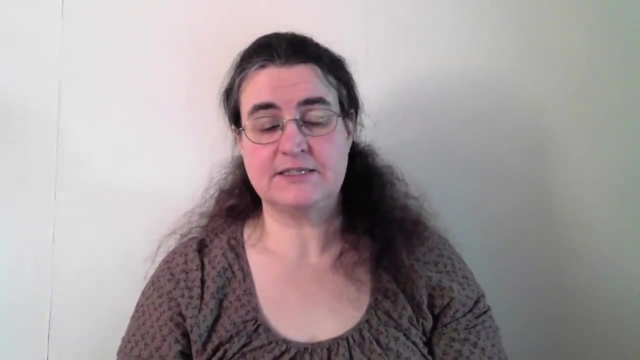 code in Idle It worked as it should. He solved this by changing the encoding. So, as we're building a search engine that will scan pages in different languages and perhaps use different language interfaces, how should we change our code so that it does? 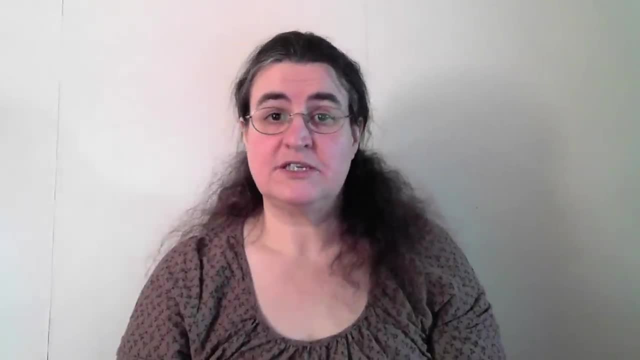 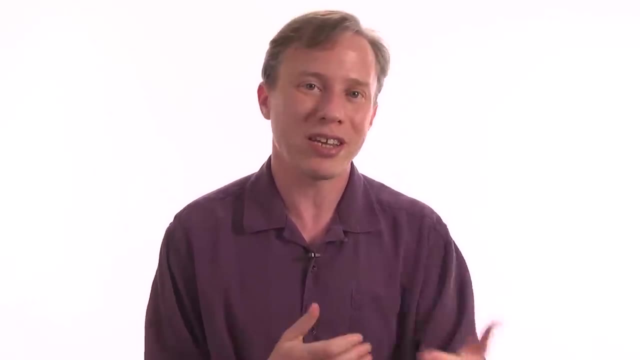 not run into problems with encoding, What should our default character set be? Thanks for the question, Raymond, And this is a really good point to bring up that. as you take inputs that include more languages than just English, well, the character sets are different, And if you look at a word like English, you'll notice that the character sets are different. And if you look at a word like English, you'll notice that the character sets are different. And if you look at a word like English, you'll notice that the character sets are different. And if you look at a web page, 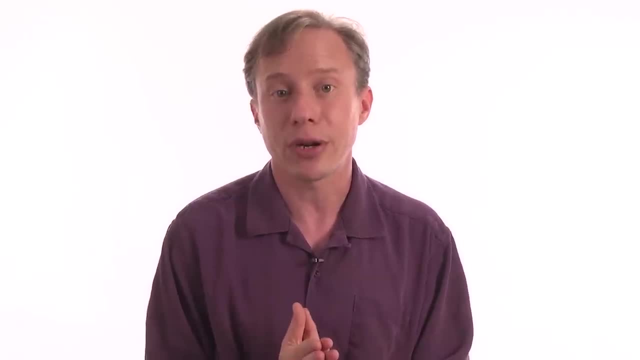 there's a header in the web page that identifies what character set it's using. This is part of the HTTP protocol: to have a header that describes the content type, which includes the character set, And the character set can be selected from a few different ones. The most common one is called 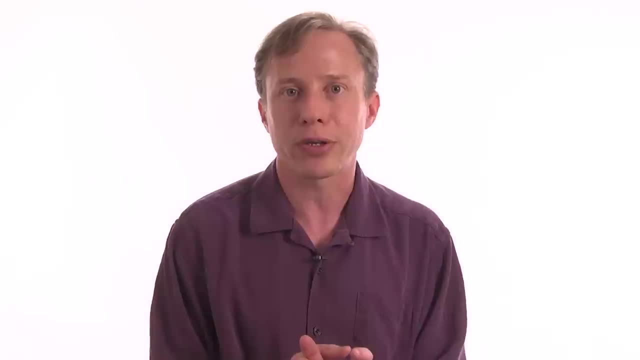 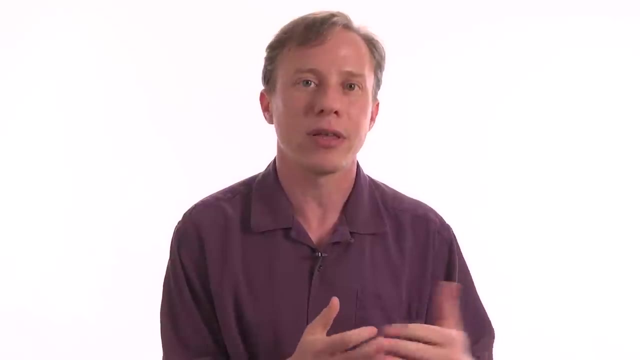 UTF-8.. And that's using a way of encoding characters that makes the simple characters that can be encoded in just seven bits, And this is the character set that is known as ASCII. these are characters that are common in English. doesn't cover all the characters that are used in 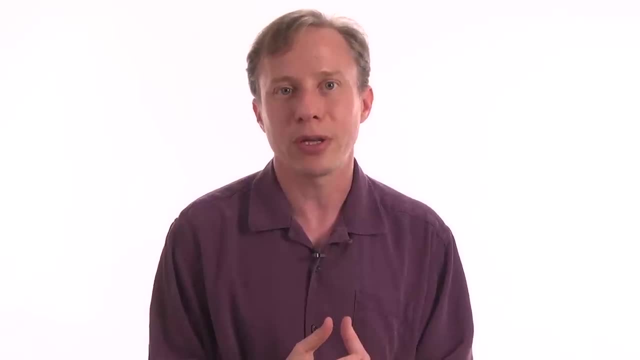 all other languages, But those seven-bit characters can be encoded using a small amount of space And the standard we've been using in Python, with standard strings that they're all ASCII, that each character is one byte. there's only 255 possible characters that can be encoded. 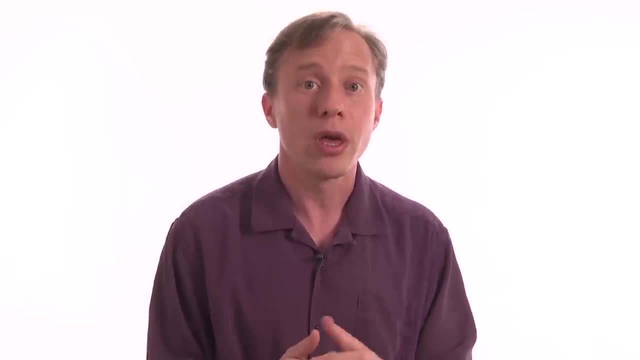 in one byte though, So if you're wanting to deal with more languages, you need to use more different characters. The way to do that is called Unicode. Unicode is a character set that that can support large numbers of characters. It's actually a way of encoding characters that. 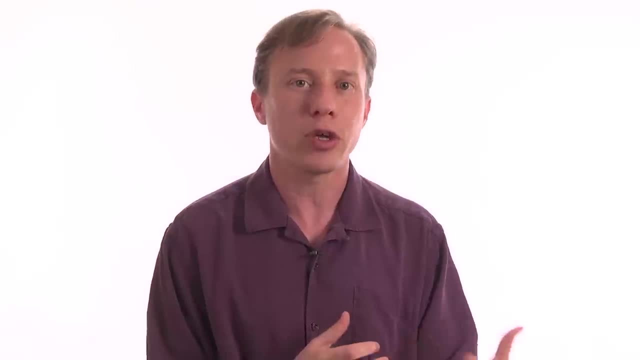 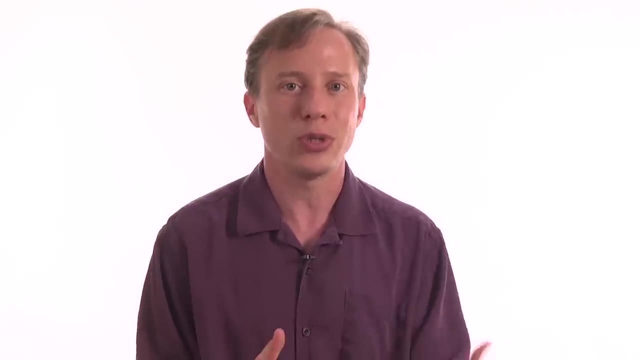 doesn't have a limit on how many characters you can support, And a way of encoding those that makes it efficient when the characters are small but allows you to still encode a large number of characters, is called UTF-8,, which is what most web browsers use To deal with this in Python.